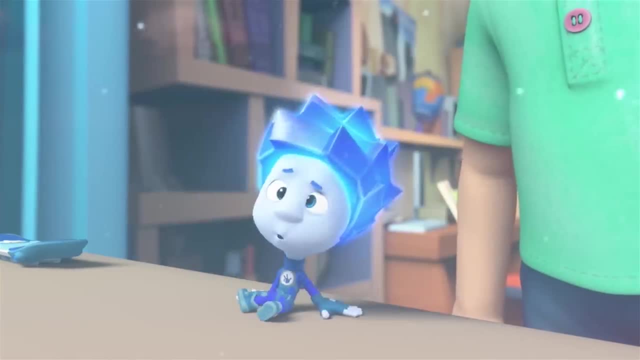 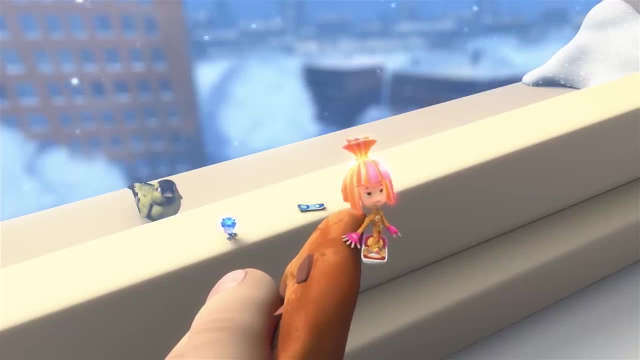 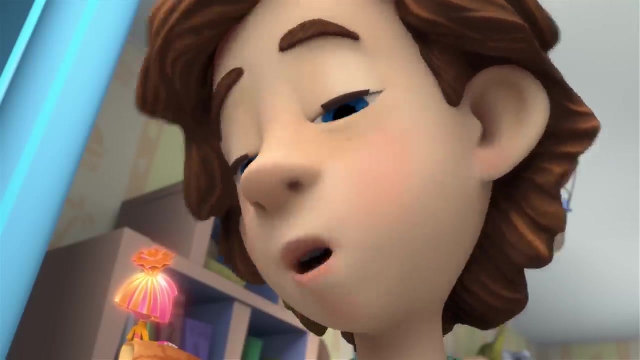 I guess he doesn't think you're funny. That's because he's cold out there. He wants to eat, that's all. Maybe we should make a feeder for the poor bird. Do you know how to make a bird feeder? No, but we both know someone who knows everything. 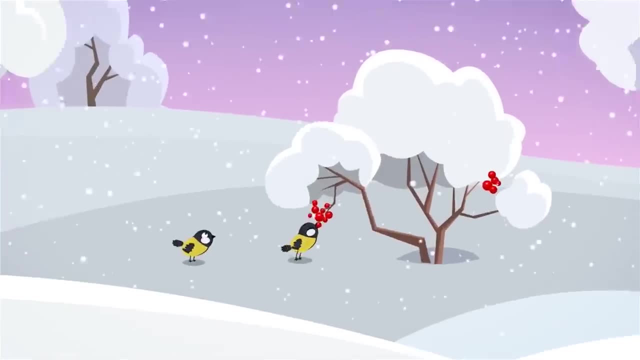 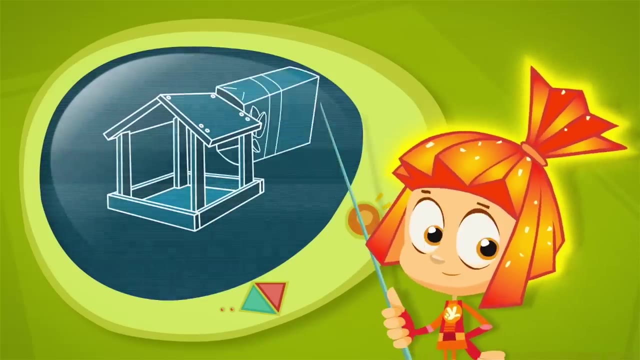 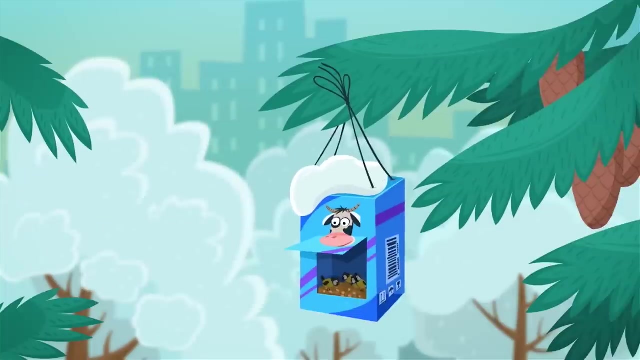 In the winter it's not easy for birds to find food under the snow. Luckily, many people come to the rescue. They build little houses for the birds, designed to hold food. The name for these houses are, naturally, bird feeders. Bird feeders can be made out of wood, plastic or even something as simple as a milk or juice carton. 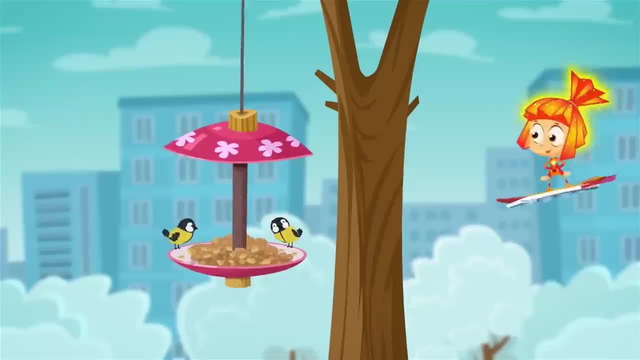 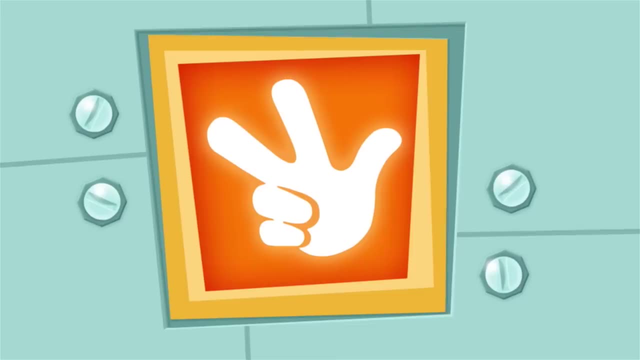 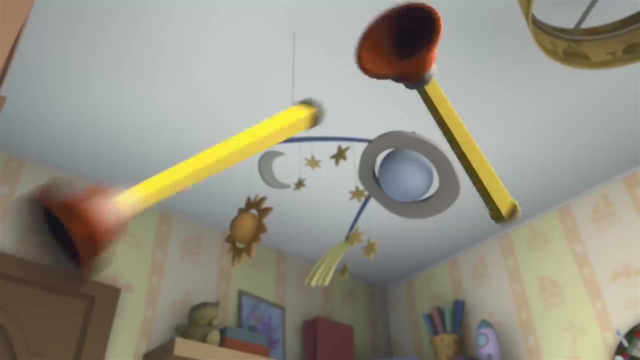 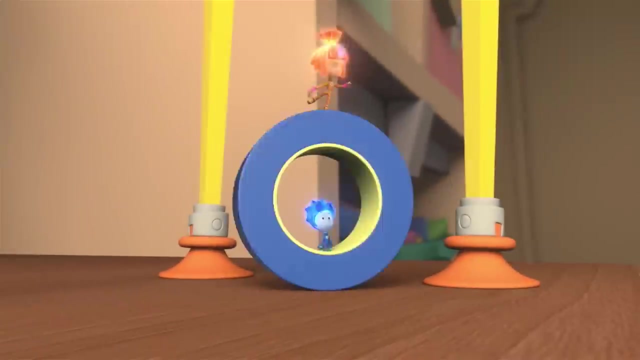 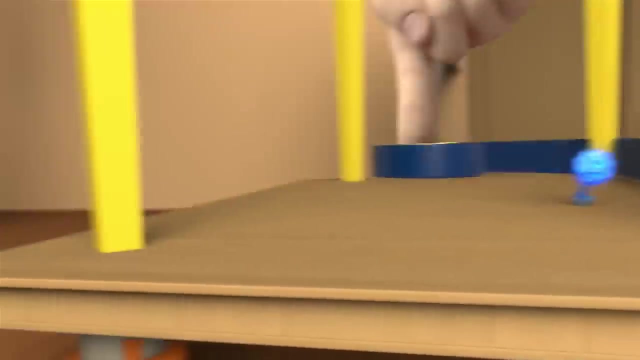 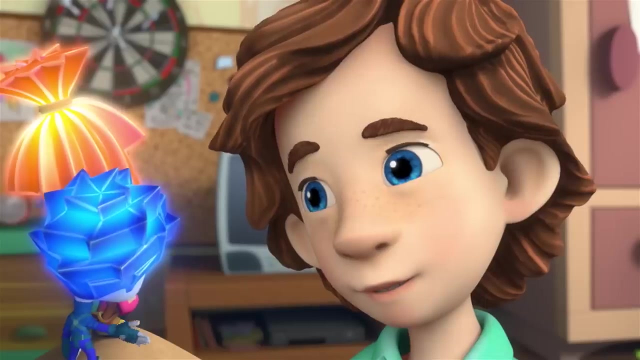 Building a bird feeder by hand isn't hard to do at all, But building it is only one part of the work. What's most important is remembering to keep it filled with food. Well, shall we start? The bird feeder is ready, And what are we going to put in it? 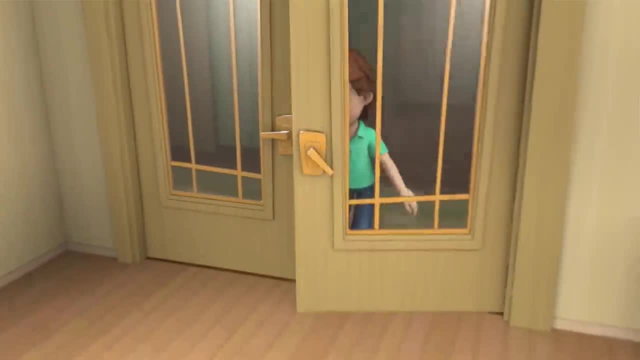 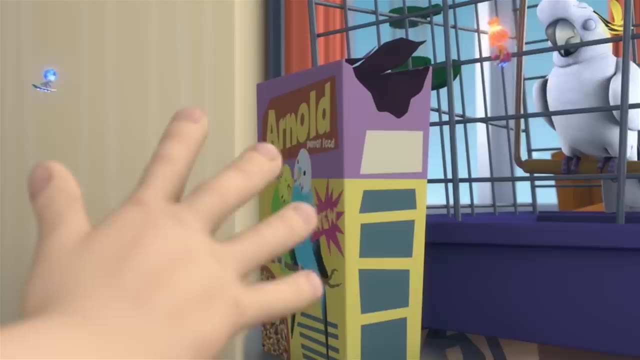 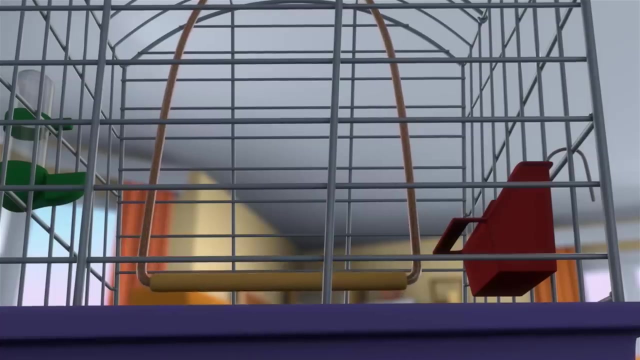 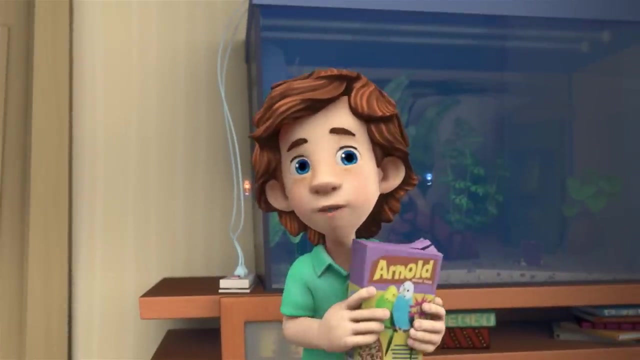 I don't know. I don't know. I got an idea. Huh, Ah, Adisa, I need some of your food for a little bird. You aren't greedy Greedy, Greedy, Greedy? I didn't know. Adisa is greedy. 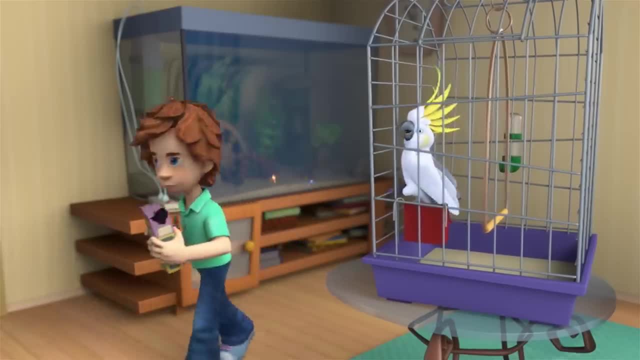 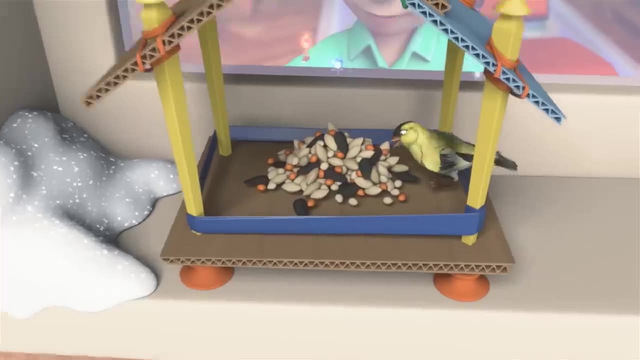 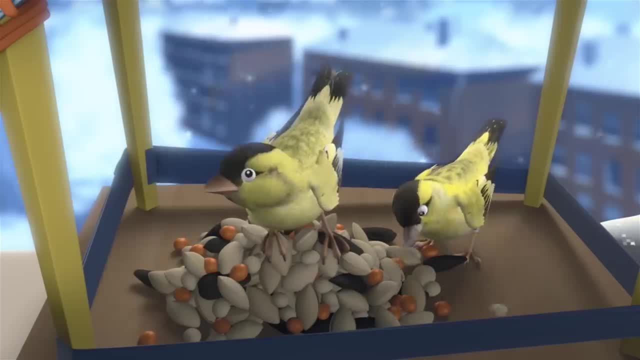 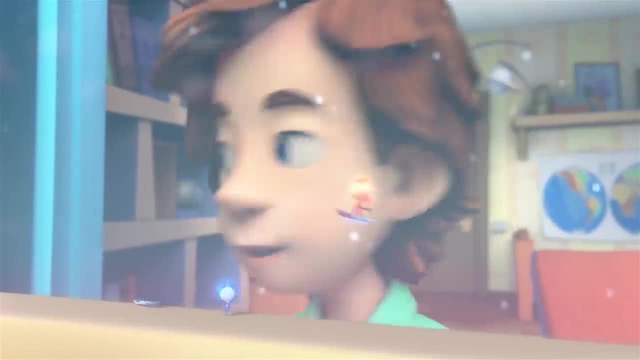 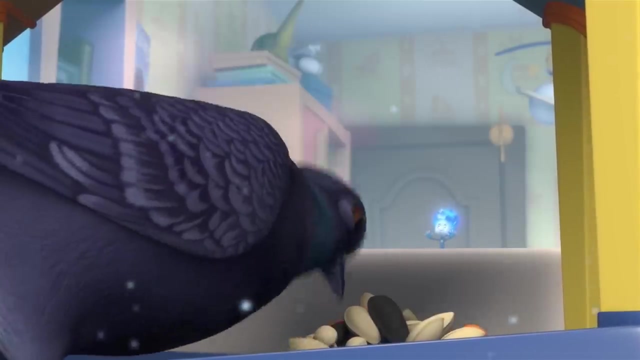 Eats. There's enough food for everybody. Poor Adisa, Poor Adisa. Let's bring them in here. We can open a restaurant for birds. Adisa's a poor little bird. Why did you scare the little birds away That feeder's for them? Get it, Just fly away. 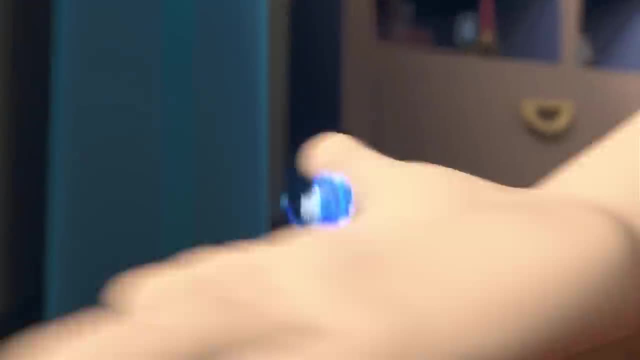 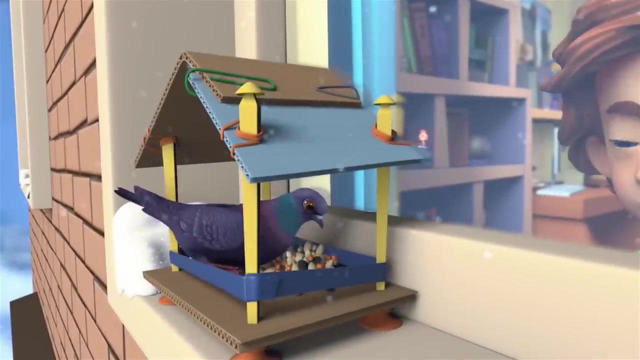 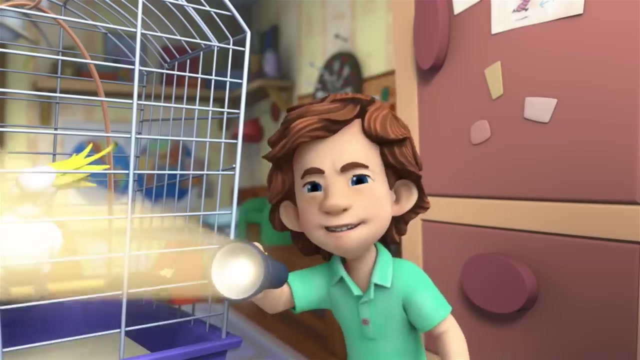 Shoot. He's bullying our friends. Hey, you leave. Leave. You'll never chase him away. now We'll see about that. Aha Serves you, right, Pigeon. It's not nice to bully little birds. It's not nice to bully little guys. 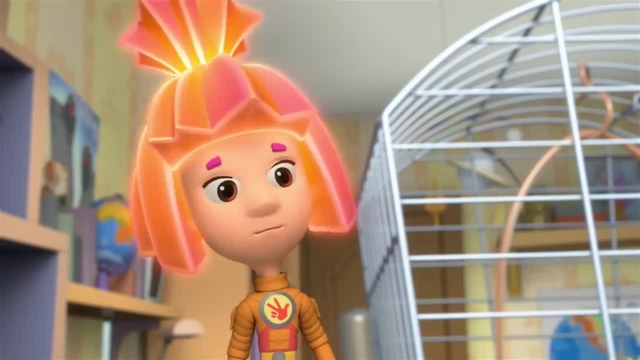 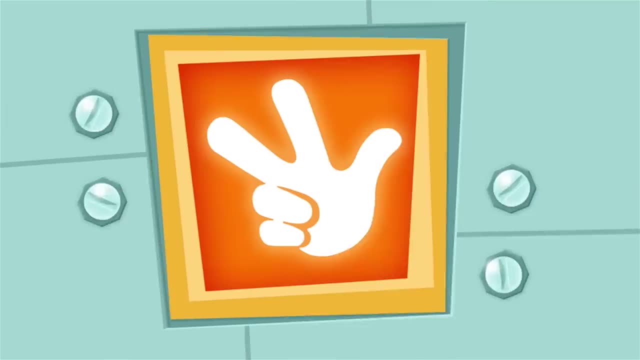 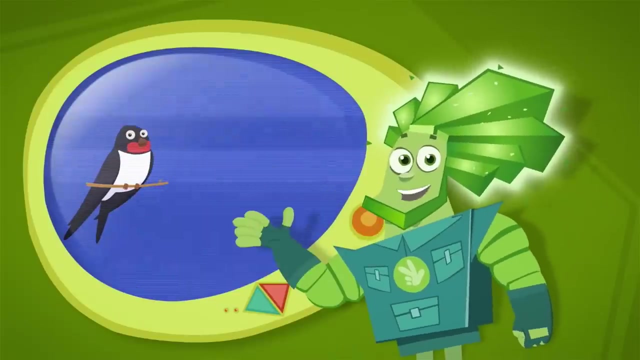 Yeah, and how about big guys? It's all right to bully them. The poor pigeon also wants some food, Food, Food, You sure? Sure, Winter can be beautiful but also very cold. Animals have different ways to prepare for when the weather gets cold. 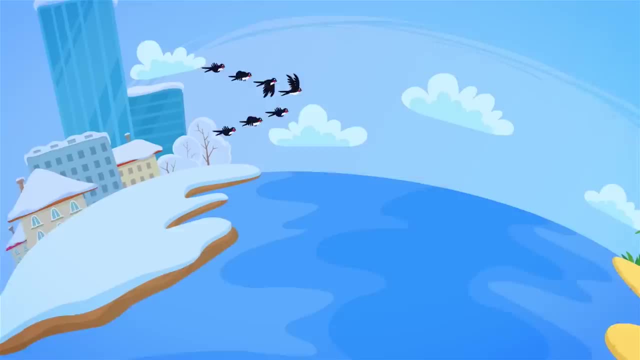 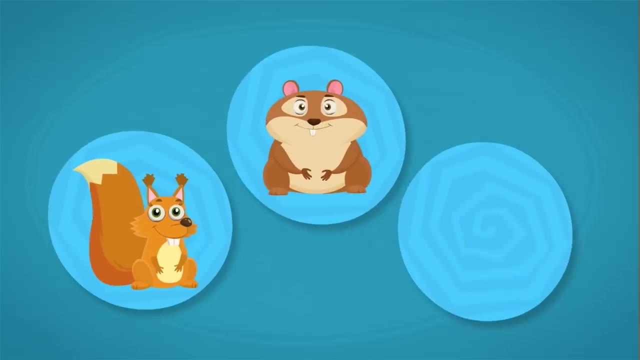 Some birds gather into flocks and migrate to where it's warmer. You could almost say they're flying to a resort. Squirrels, hamsters and chipmunks collect and store nuts, mushrooms and pine cones. There are many people who don't have pantries that are as well stocked. 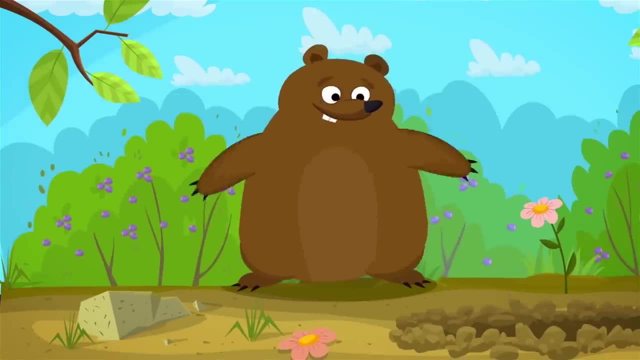 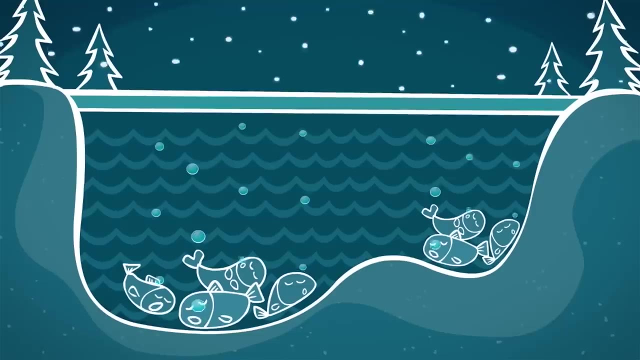 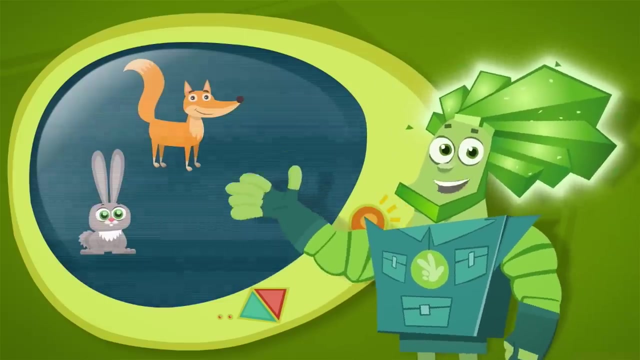 Badgers and bears eat a lot of extra food in the fall and then go to sleep in their dens and burrows for the whole winter. Fish also sleep in the winter, only they're at the bottom of rivers and lakes. Frogs, snakes and even wasps burrow in the ground while hares, foxes and wolves grow thick coats. 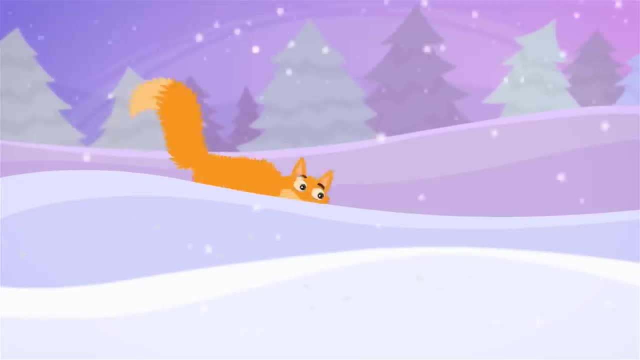 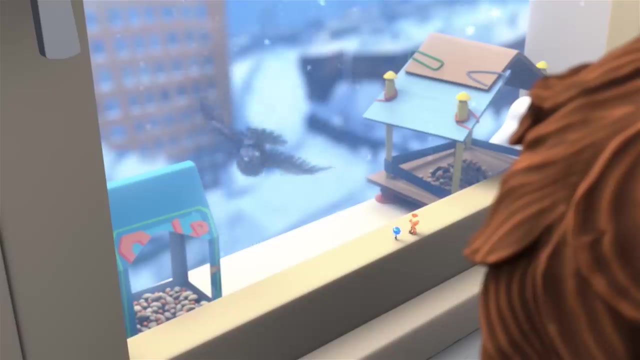 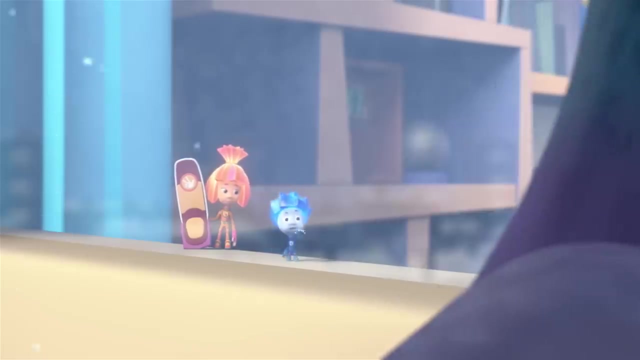 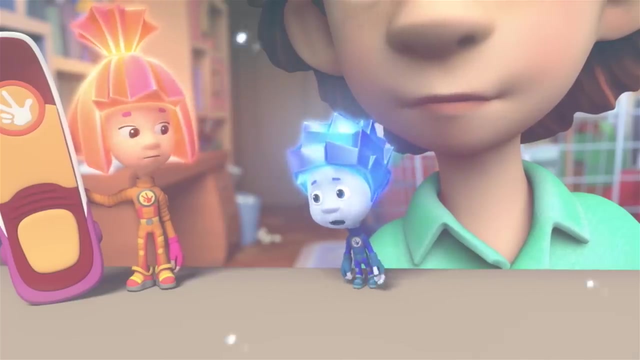 that protect them from the freezing cold, Although it isn't easy for them to find food. So that will be your feeder and that new one will be for the little birds. Hey, are you taking their food again? There you go, But those little birds, they'll probably never come back here. 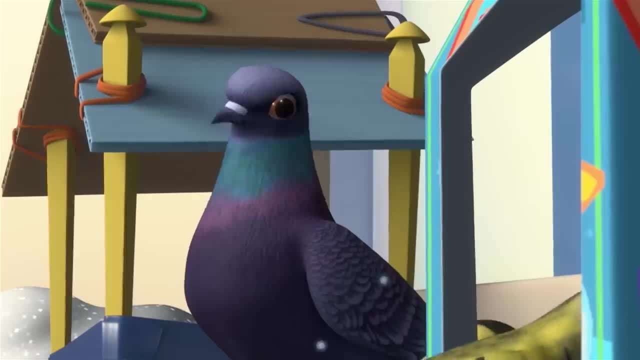 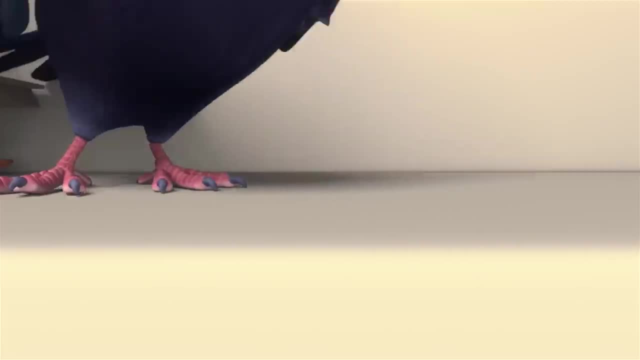 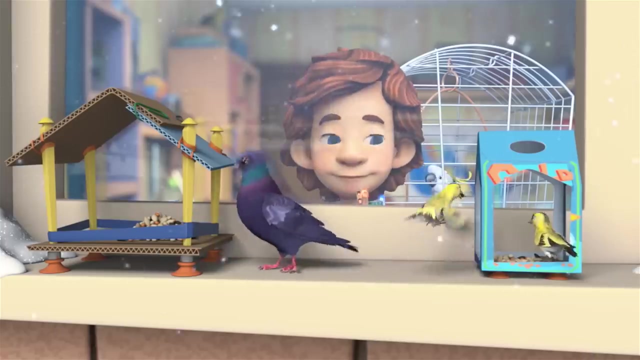 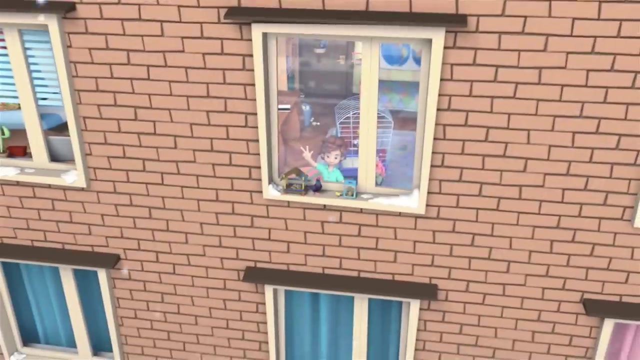 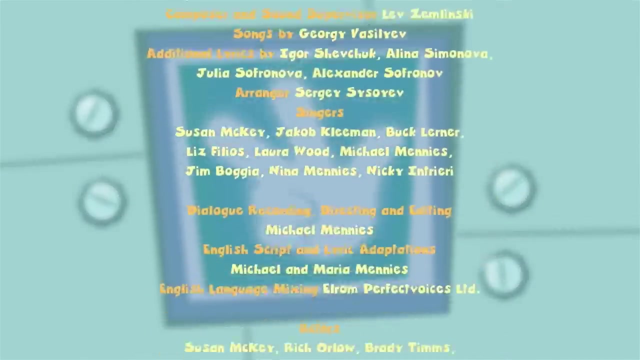 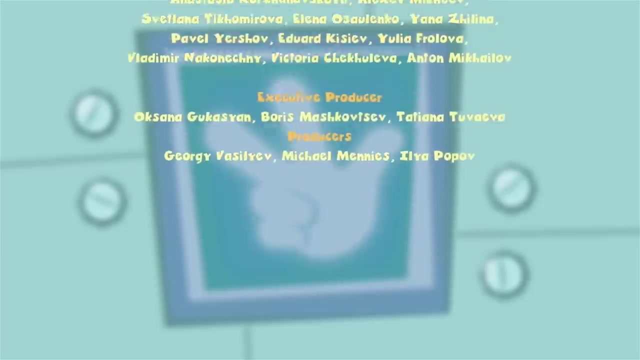 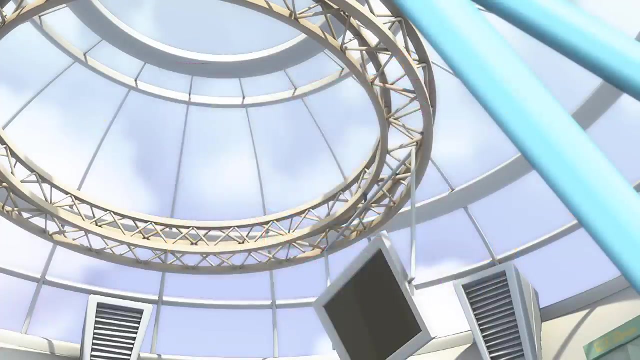 Look, Nolik, They came back, They're here. Aww, they're full and happy. It's so nice. Tideesh, Tideesh, Zip, Zip The Drum. Now let's turn it on. It's buzzing, You hear it? 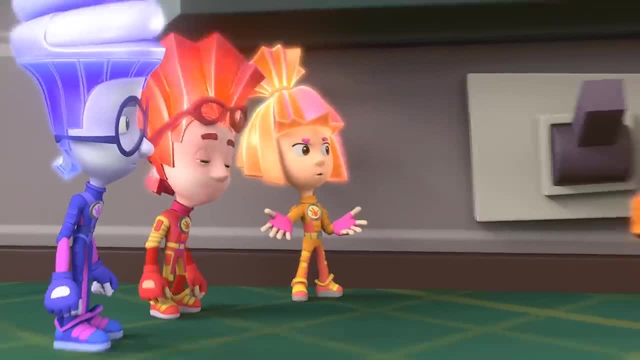 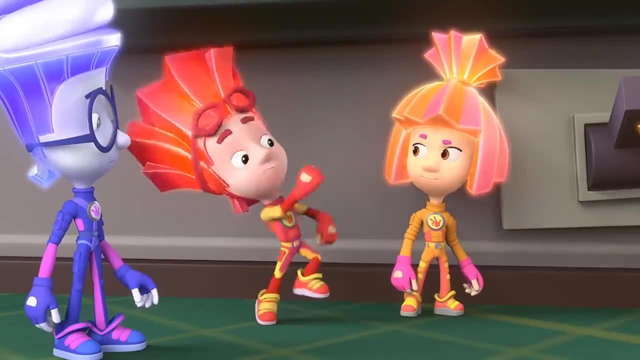 I would love to, But the only thing I can hear is Nolik's banging. Nolik, what are you doing? I'm rehearsing my solo. Nolik's the drummer in our rock band, Didn't you know that? 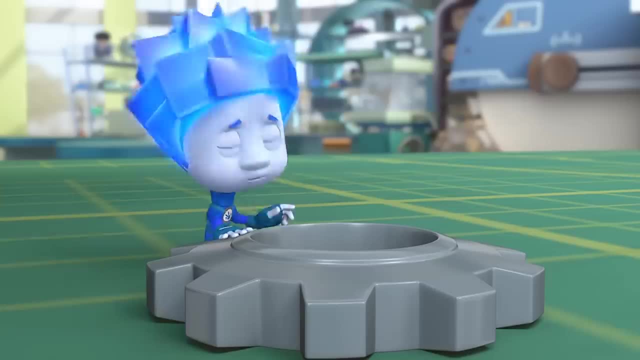 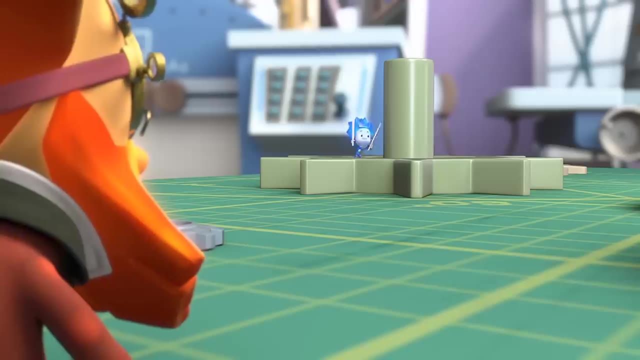 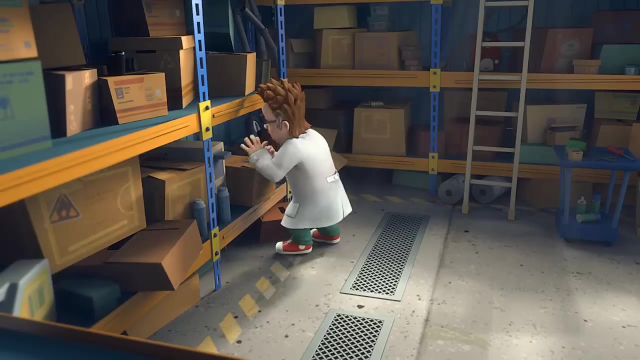 Why don't you go and rehearse somewhere else if you wouldn't mind? Yeah, alright, I just can't work like this. Nolik, stop it please. Oh, my head is just spling. Professor Eugenius, will you come to the laboratory? 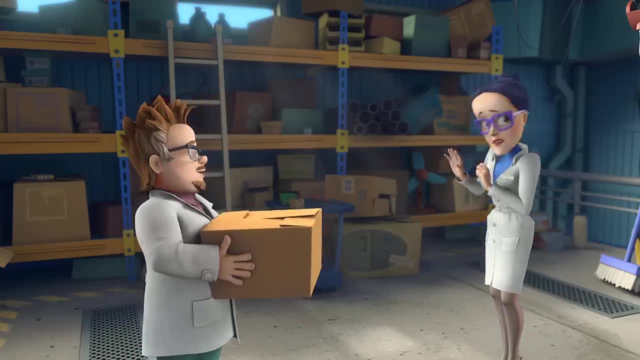 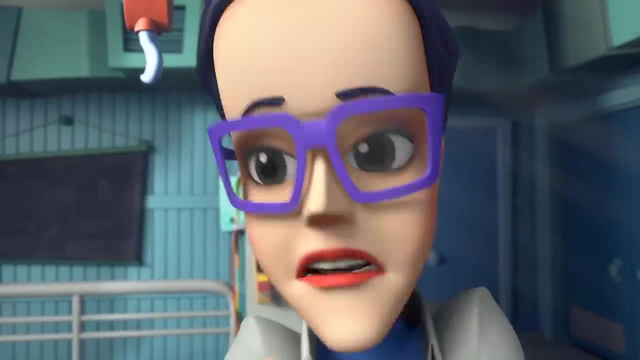 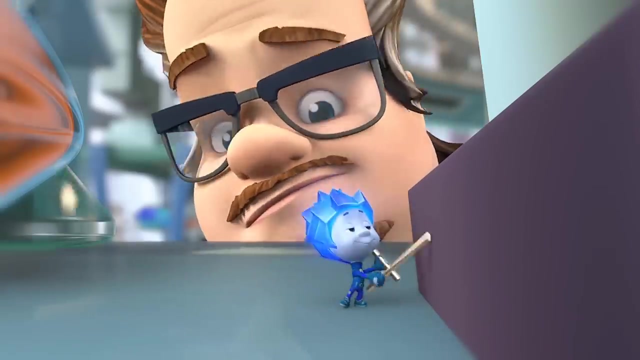 There's something very strange in there. What I'm hearing? some kind of awful sound. You are, I think it's a ghost Back from the dead. Don't you worry about ghosts, Lisa, I'll check what it is. Hmm, so it's you making the racket. 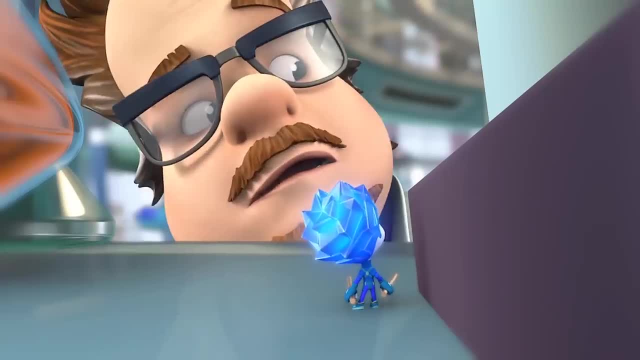 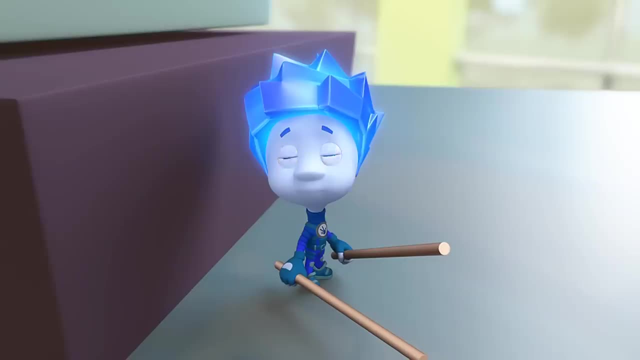 What I'm just rehearsing. Well, what is it? Don't worry, it's just a piece of equipment rattling. You know what you should do. You should go and practice back at home. my young friend I know, but I don't know how to do it. 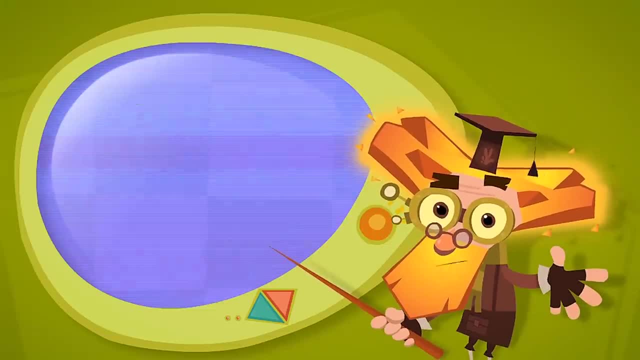 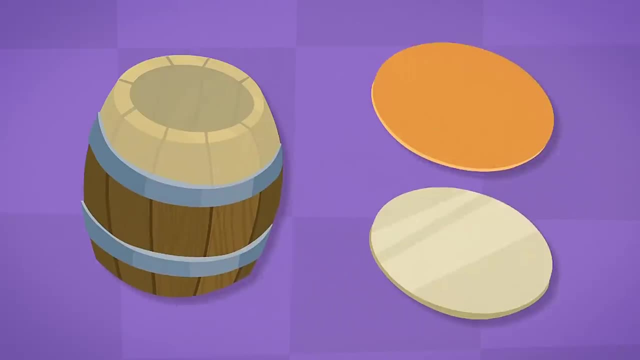 I don't know how to make a drum. It's not very hard to make a drum. One way to make it is to take an empty barrel and replace its bottom with a skin made of leather or plastic. If the skin is stretched tightly, the sound can get very bright and loud. 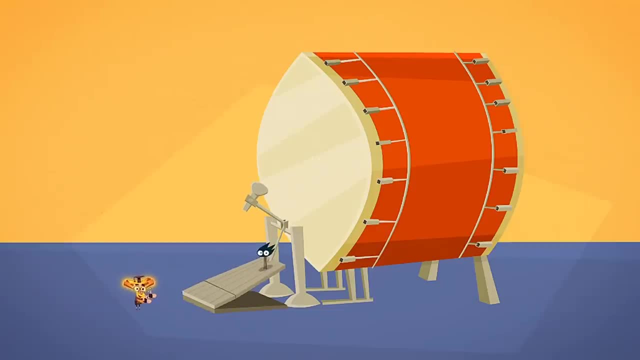 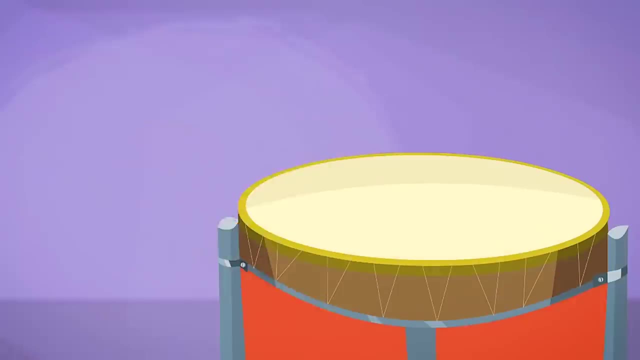 Really big drums are usually played with percussion mallets or beaters, while smaller drums can be played with sticks or with bare hands. Instruments that make sounds by being shaken, scraped or beat. Instruments that make sounds by being shaken, scraped or beat. 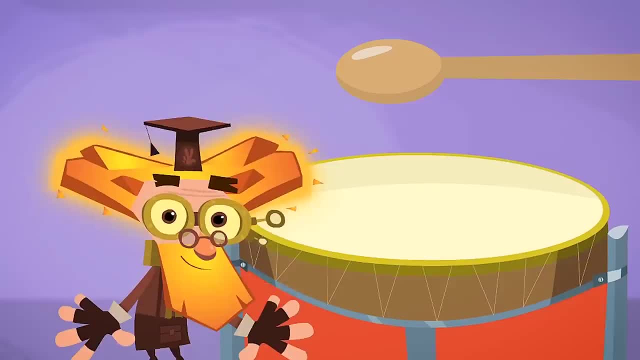 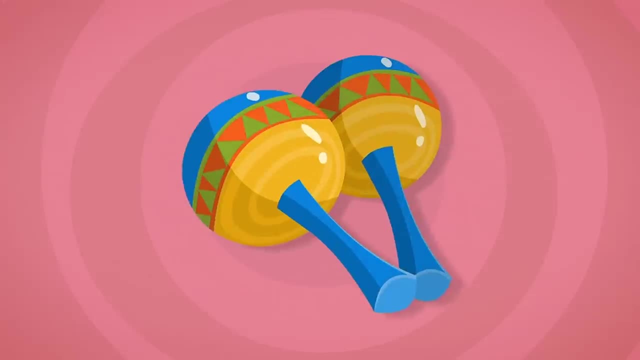 Instruments that make sounds by being shaken, scraped or beat are all called percussion instruments. There are lots of different percussion instruments, Like the small hand drums that are called bongos, Big shakers with handles called maracas Cymbals made out of metal. Now, those really make a lot of noise. 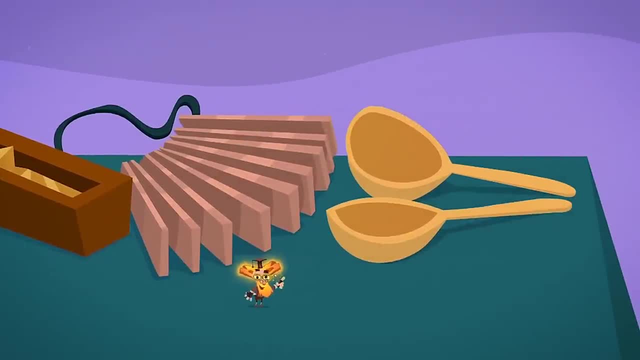 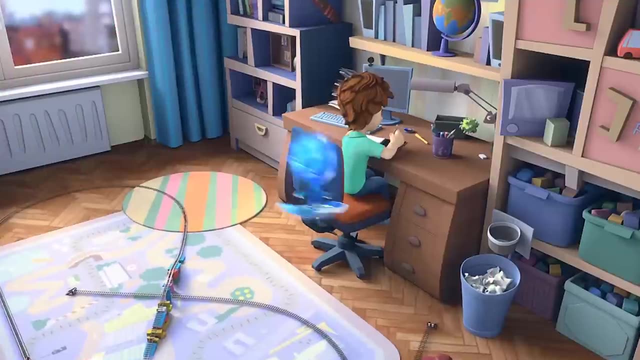 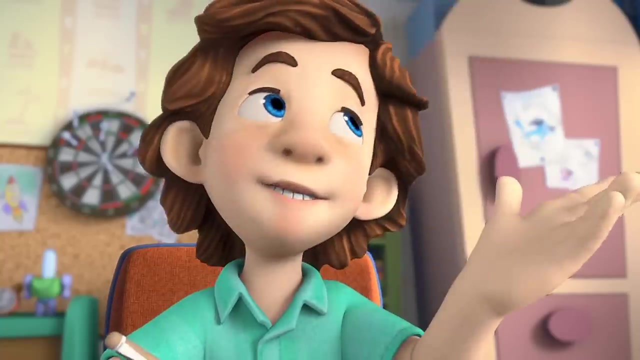 And there's tambourines, ratchets and even spoons. That's right. People can make music using spoons as a percussion instrument. Tom Thomas, Do you think I could practice my drumming here? Yeah, Go ahead. I've just got some homework to do. 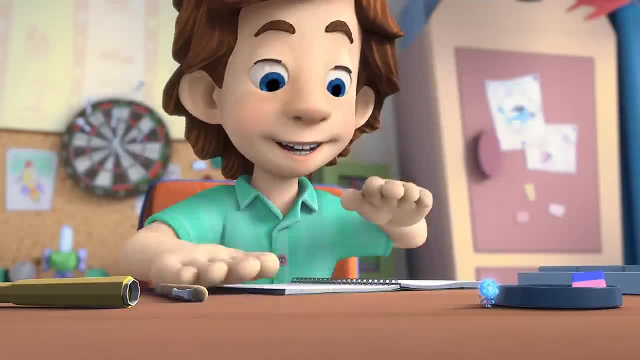 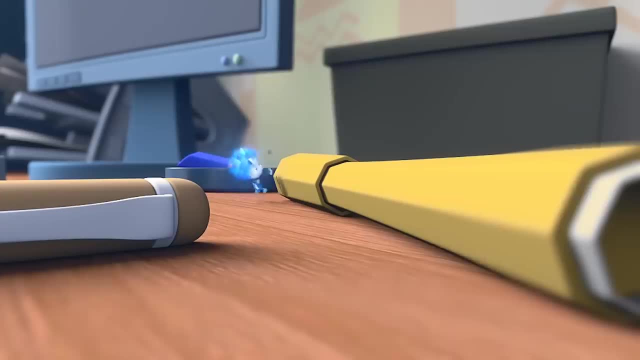 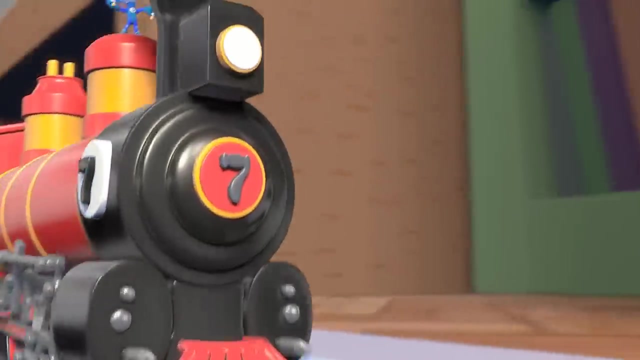 I can do that, And better than you can too. And what if I play like this? huh, Then I'll go like that Or like that, Ever since I had decided That a drummer's what I want to be. There is nothing That I won't bang on. 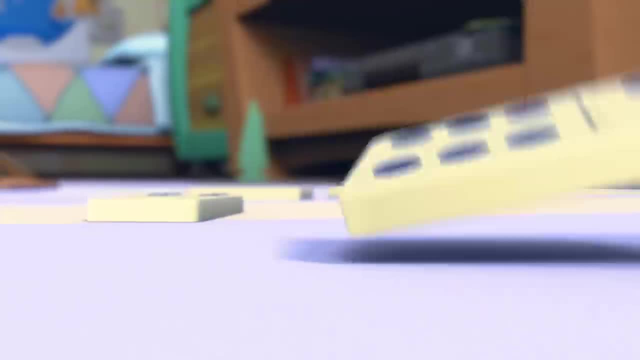 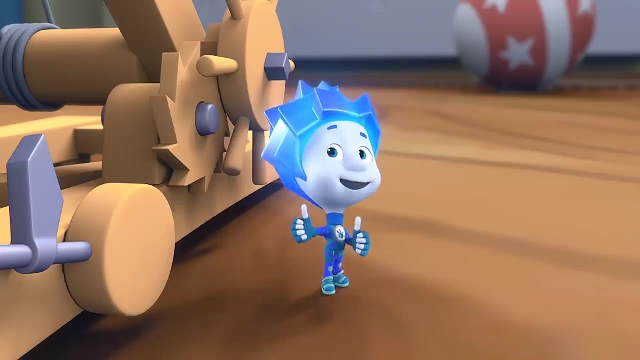 Cause the world's a drum to me. So I bang On radiators With a spoon. The pot goes Boom, bam bam. Maybe someone Will take pity And they'll buy me My own drum. Bang it, bang it, bang it, Boom, bang it, boom. 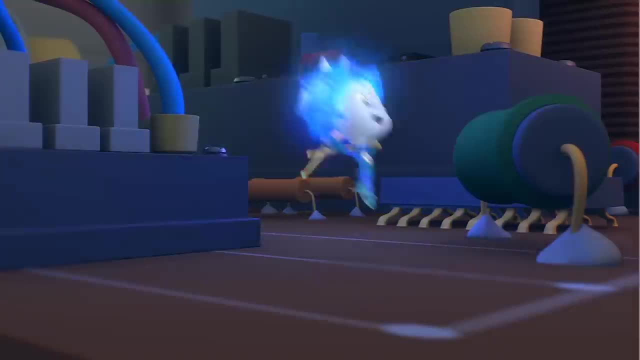 Bang it, boom Bang it, bang it, bang it, Bam bang it, bam Bang it, bam Bang it, bang it, bang it, Bum bang it, bum Bang it, bum Bang it, bang it, Boom, boom Bang the drum. 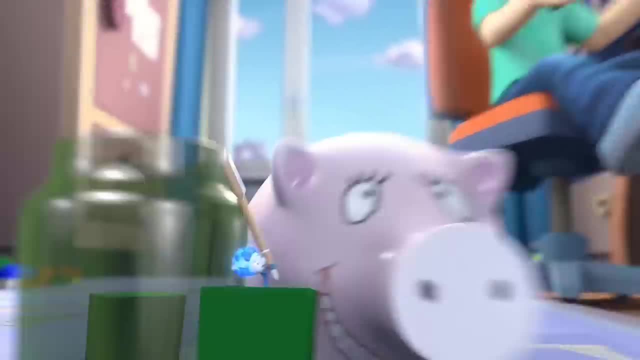 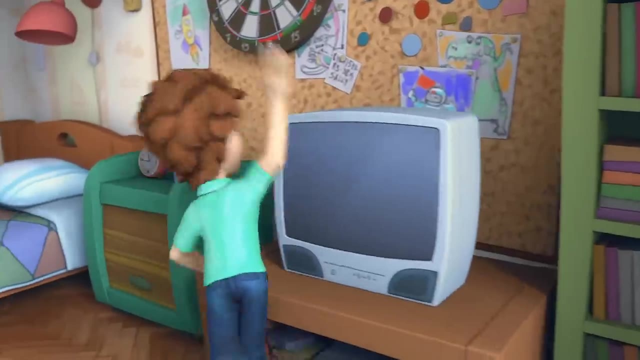 Bang the drum, Bang the drum. Both my father And my mother Wish I'd play A violin instead. I don't want to. I'm a drummer, But I can drum That in their heads. So I bang On radiators With a spoon. The pot goes Boom bam bam. 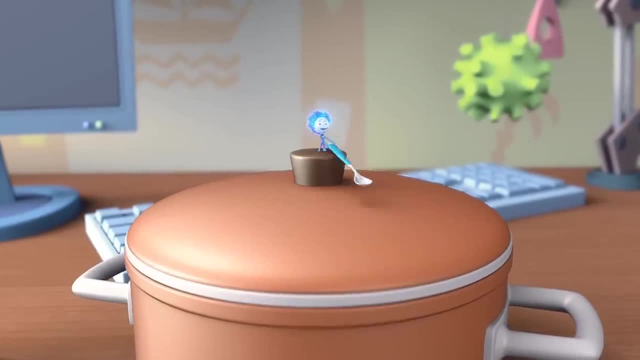 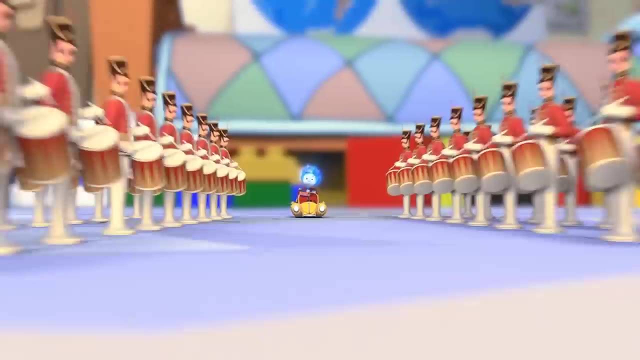 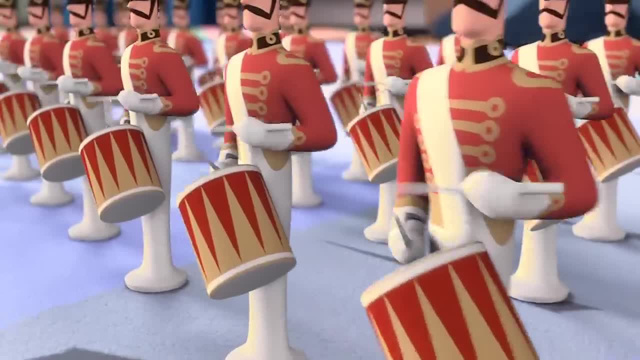 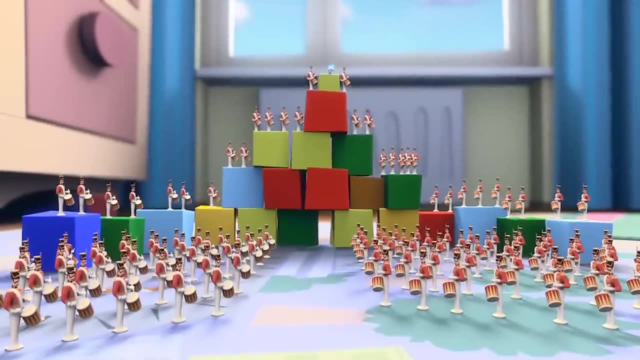 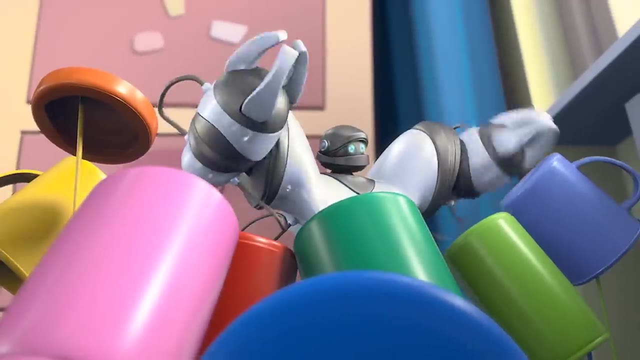 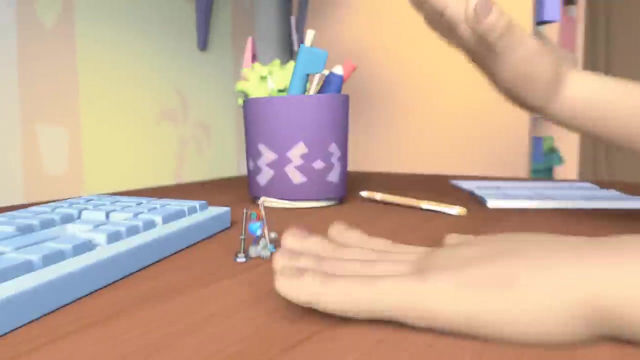 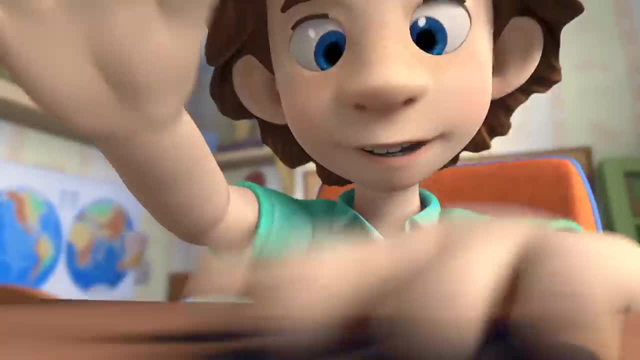 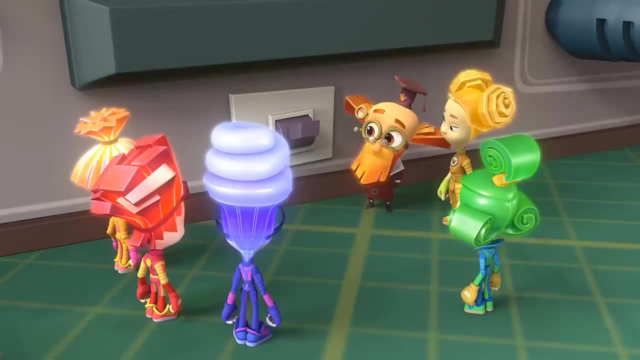 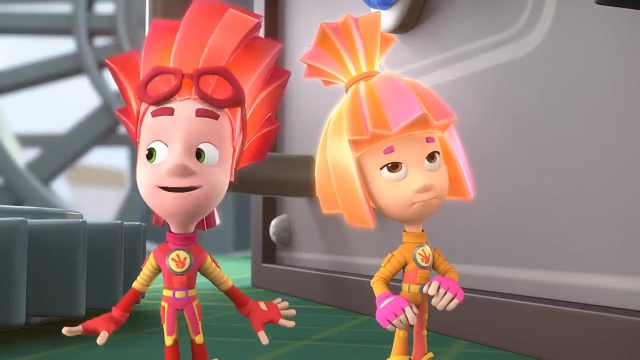 This is fun. Maybe it's fun for you. Bang the drum, drum, Stop. That's enough. Bang the drum And now let's turn it off. Can you hear that It stopped buzzing? It did, Hey, everybody, it's Nolik Yo, What's up?